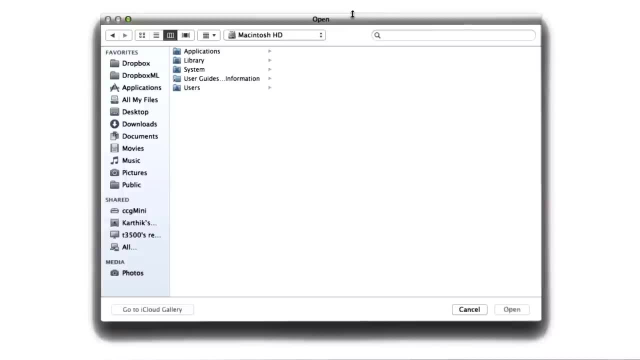 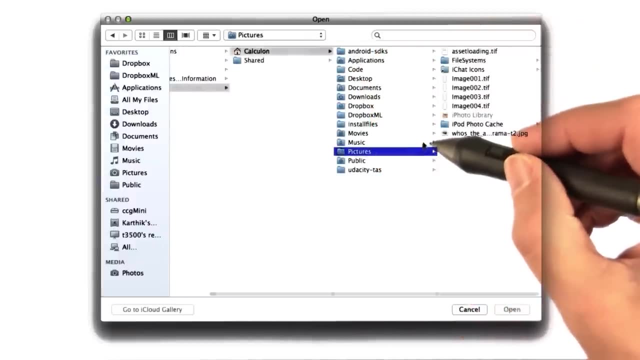 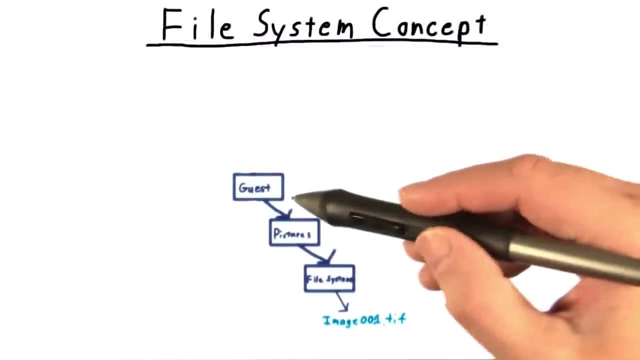 Most any time that you use a computer, you're going to interact with the file system. Here you see me navigating the file system on my computer to find this presentation. There it is. I started off in my home folder. Inside of there I went to pictures and then to file systems. 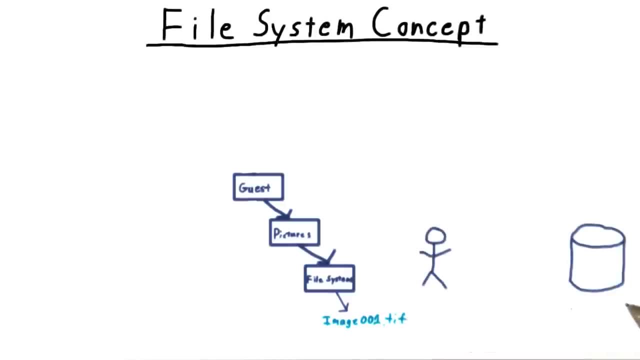 And there I found the image that I was looking for. This is really convenient. In my case, the data I was looking for was on the hard disk on my local machine, But I didn't have to remember physically where the data was, ie the platter, the track, the sector number. 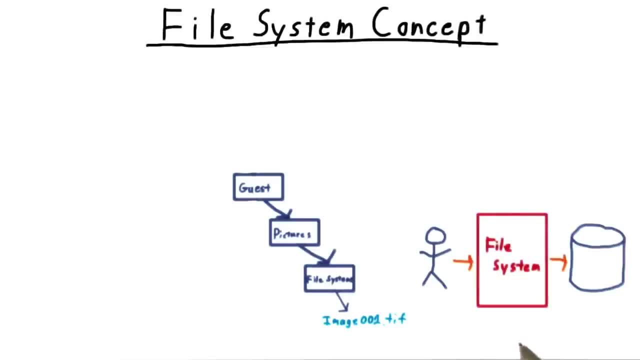 etc. Instead, I was able to access the data through a very intuitive interface provided by a file system module of the operating system. There are at least three key abstractions at work here. The first is the notion of the file itself. In reality, the data may not be placed next to each other on a disk. 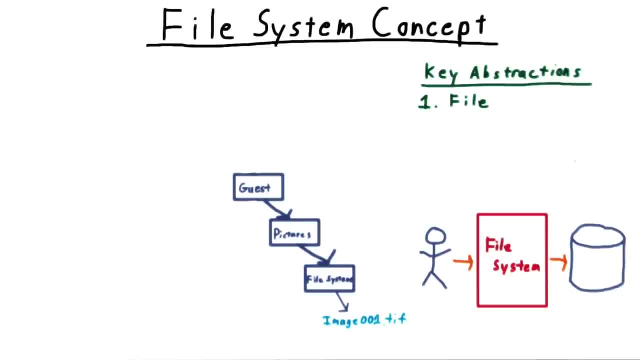 all in the right order, But an application developer- the author of the sketchbook program I'm using, for instance- gets to create the data of a file as one big, long, contiguous string of bytes. Second is the file name. I don't have to remember any of the physical. 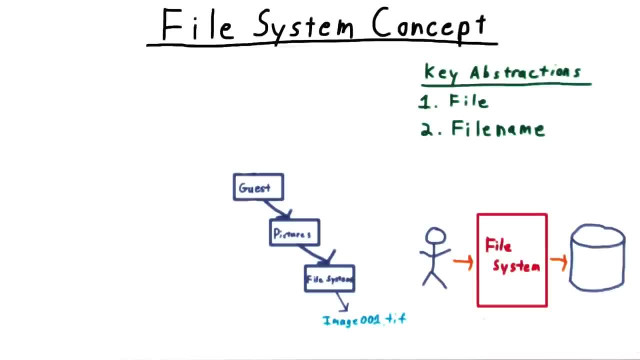 information about how my file is stored, the sector number where it starts, for instance. Instead, I get to assign my file an intuitive name, in my case image001.tiff. Third is the notion of folders, or directories as we will call them. These are containers for other files or 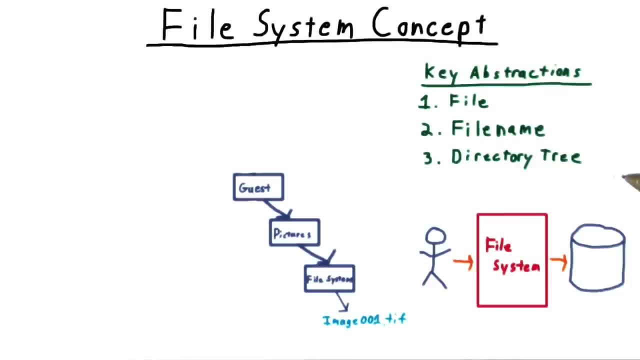 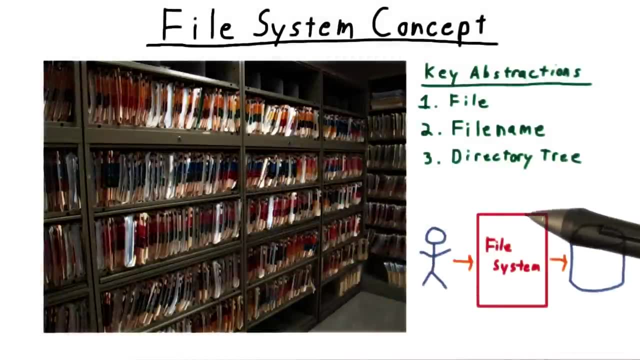 directories that help keep things organized. The idea is that we have an electronic version of what was once the more common physical filing system. We put folders within folders to help us keep things organized. So on this machine then I don't just have a pictures folder but also a documents folder, And within 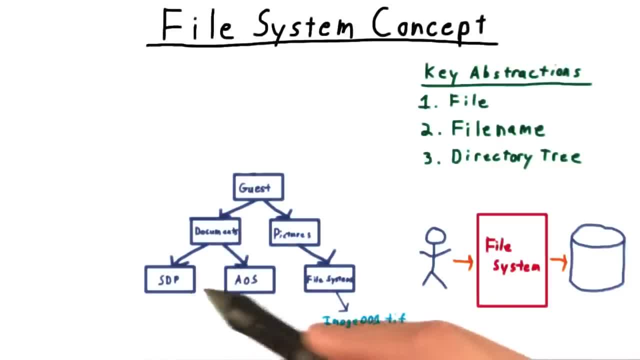 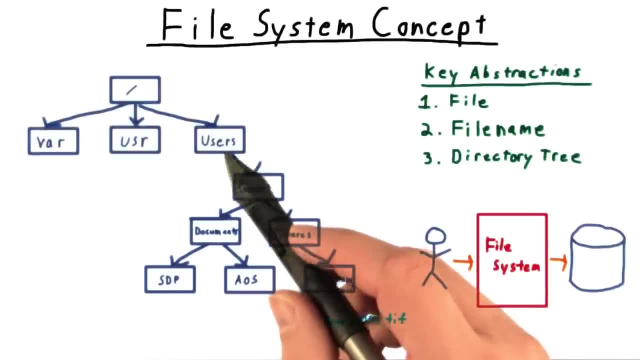 there I have a folder for advanced operating systems and maybe there's another one for a software development process, etc. And even this home directory sits inside a larger directory for all users, which then sits inside of a directory called root, which then contains folders for the operating. 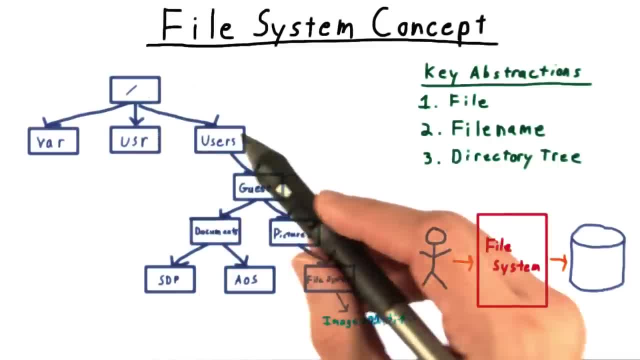 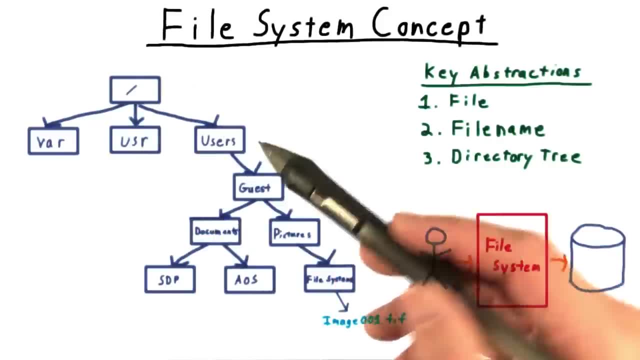 system and other things. It's called root because if we think of this directory structure as an upside down tree, then this all encompassing directory would be the root, or the base of the tree. Indeed, the structure will always be a tree, just by.